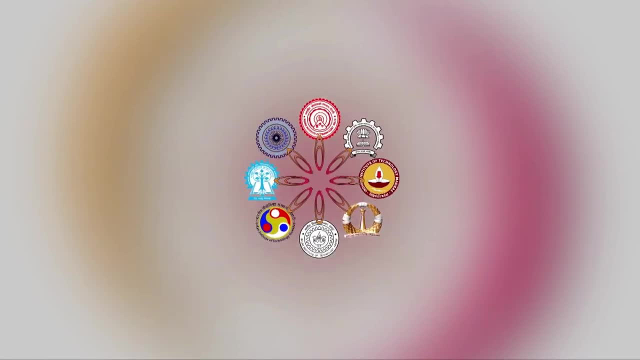 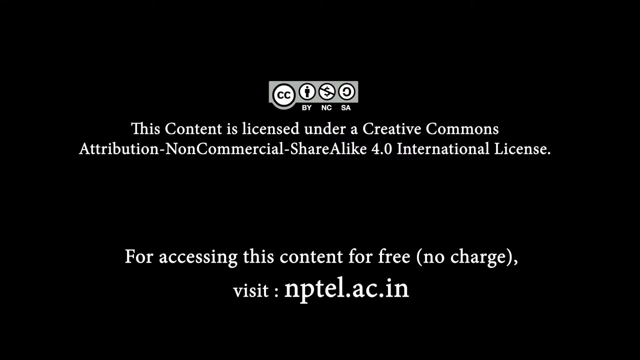 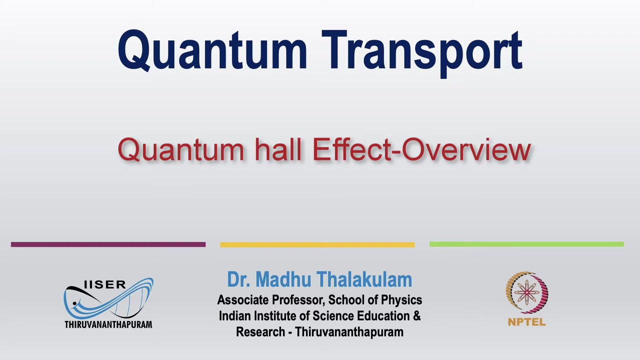 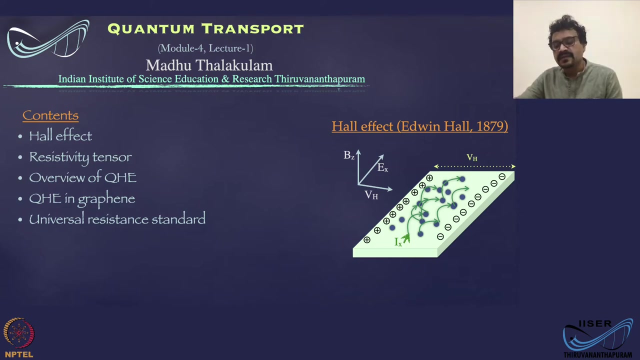 In this module we will start discussing a touchstone quantum phenomena or two-dimensional system, that is, the quantum Hall effect. So before we dwell into the details, let us quickly and briefly review the classical Hall effect, which was discovered by Edwin Hall in 1879.. So what you have here is you have a conducting material and you have a magnetic. 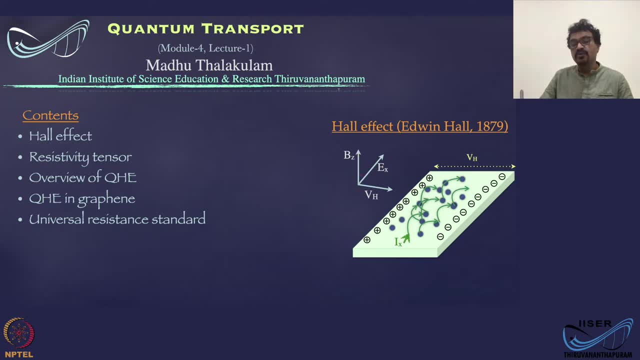 field which is applied to the plane, normal to the plane, and you have an electric field along the plane of the sample And the transport of electron is driven by lot of collision process as described by the two pictures, two spheres. Now the electron will undergo cyclotron motion, But at the same time electron will 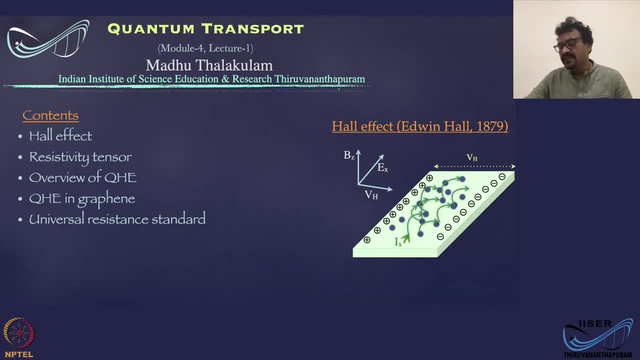 undergo many collisions and eventually the electrons will get deflected towards the, towards one end of the one edge of the sample And other edge, you will have the positively charged ions And at some point of time a balance will be reached by the, by the electron. 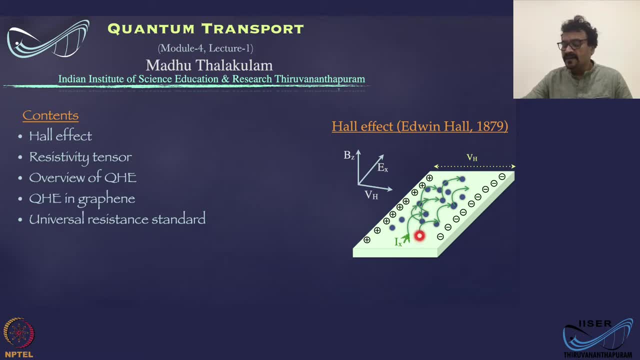 applied by the field generated by the exposed ions and the collected electrons, and no more electrons will be actually collected and there will be a steady state where a voltage is generated across the edge, that is, the D H, the Hall voltage, and from this Hall voltage we can get information on the carrier. 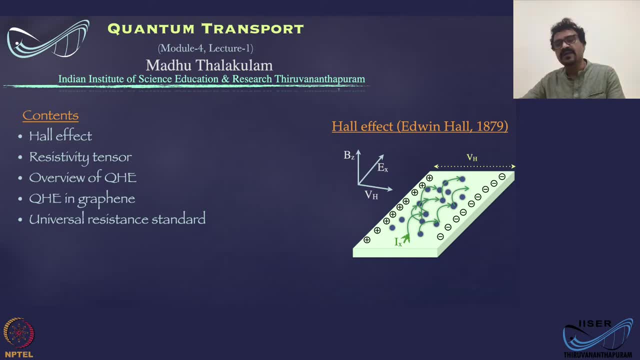 consolidation in this, in the sample, and we can also extract other from the carrier consolidation. we can extract mobility, conductivity and all these details. okay, now in this lecture we will briefly we will go through the mathematical formulas of the quantum of the Hall effect briefly. then we will define the resistivity tensor and overview the 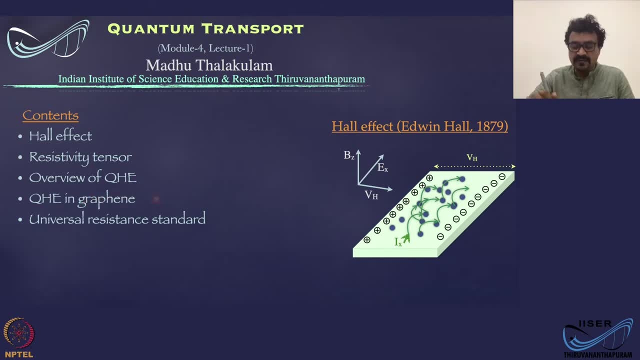 quantum Hall effect and we look into the quantum Hall effect in graphene and how the quantum Hall effect is used as a universal persistence standard. so that is the plan for this lecture. okay, in the next lecture we will look in the mathematical formulism of the quantum Hall effect. how do, how are we getting? 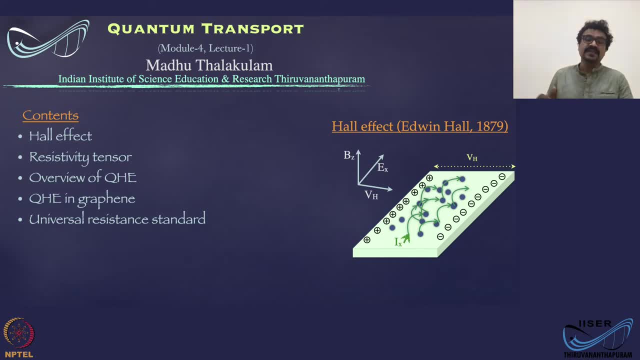 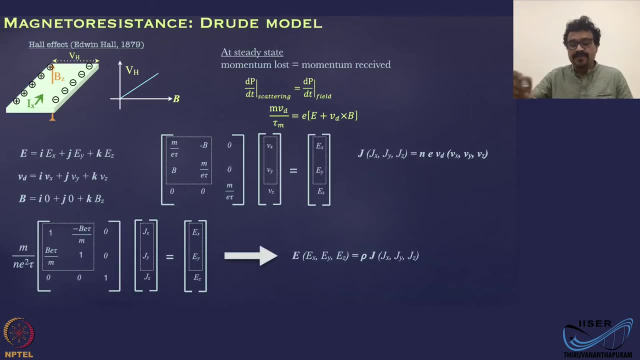 the quantized persistence andstory. all those details in the coming lectures. ok, Alright, so this is the picture of the sample, where we have a magnetic field which is applied perpendicular and there is an electric field which is driving the current Ix. ok, And the quantum Hall effect actually is slightly different. 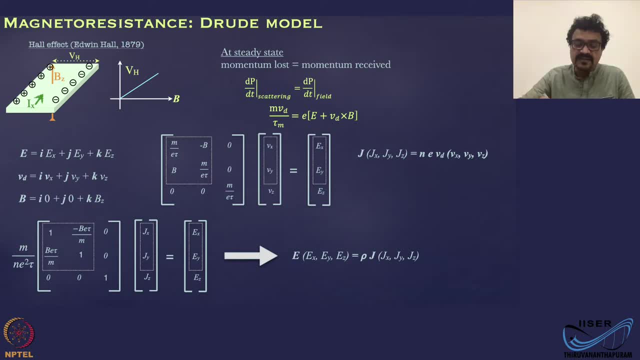 that applies to a two-dimensional system, but in this case we are considering it is a three-dimensional material. ok, In the normal Hall effect, what you have is you have a B field and you are plotting the Hall voltage or the Hall resistance. If you divide the Hall voltage by the 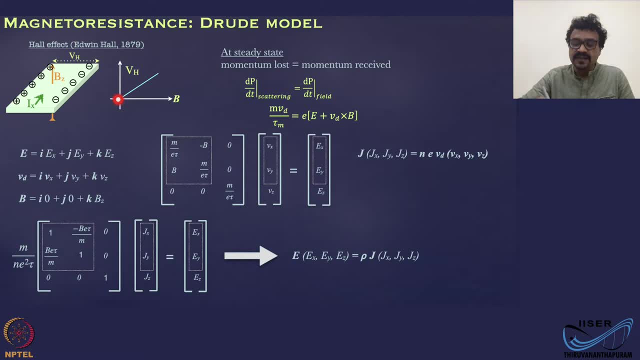 current, then you will get the Hall resistance, then you will get a straight line, that is, the Hall voltage is proportional to the B field. Now the assumption is that the current is a three-dimensional field. ok, So the assumption here is: the carriers undergo scattering with. 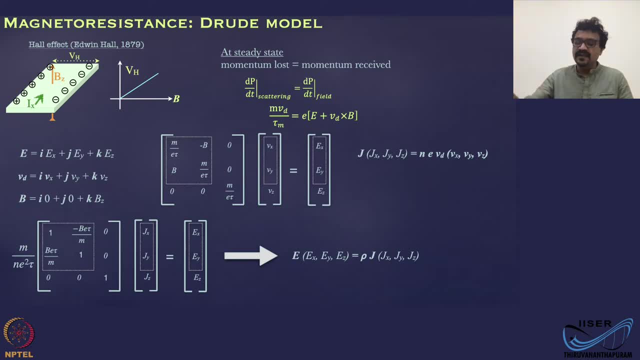 various scattering suggestions at the material, and the momentum lost during the scattering is actually momentum received from the field and this is the condition for the steady state. And you have the E equation of motion here. this is the force: m Vd by tau, m ok Vd is the drift velocity. 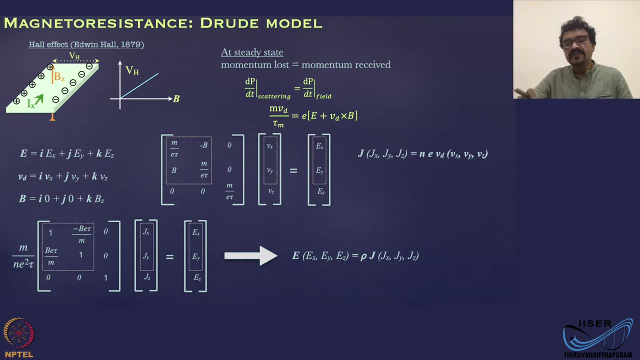 tau m is the scattering time, or that is the force experienced by the charge carriers. ok, And there is a force exerted by the electric field and this is the force by the magnetic field: v, cross, B term and E. this is the force to the cross field. So this is the force. 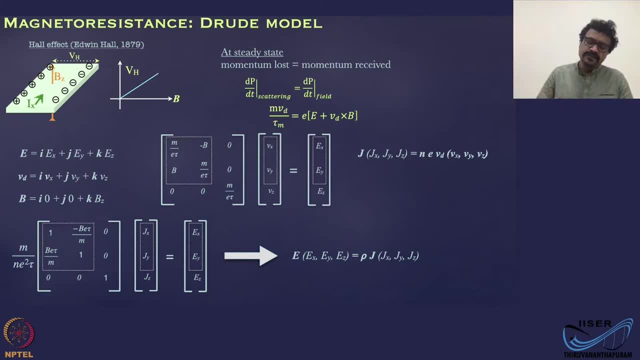 to the cross field. Now, what we are doing here is we are going to look into the action in terms of the various components of this field. We have field separate into the xy and z component, The velocity, the drift velocity, vx, vy and vez, and the B field, which we have played only in one direction. 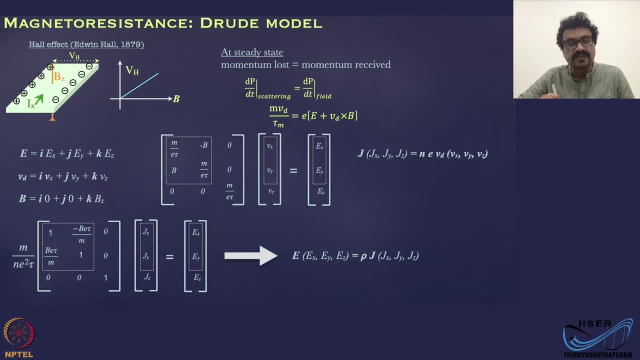 that is the vz- into the x and y. But what we are going to do now is we are going to set- that is the only component I am going to consider- ok, And once we substitute these three in this equation, you can generate this matrix. ok, So I have marked a small square. 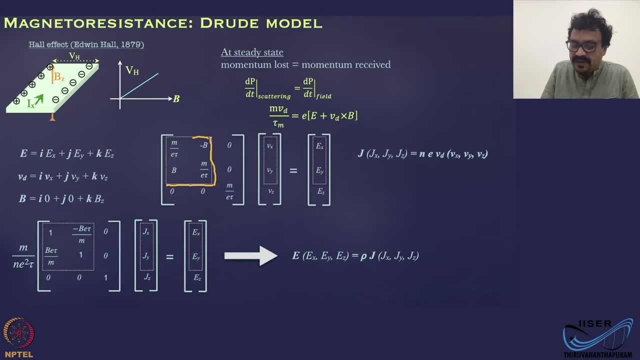 matrix inside this as 2 by 2 square matrix inside this. that is what is going to be relevant for a two-dimensional system Eventually. that is what is going to decide the whole voltage and whole effect, because the moment you apply magnetic field, all the action of the electron 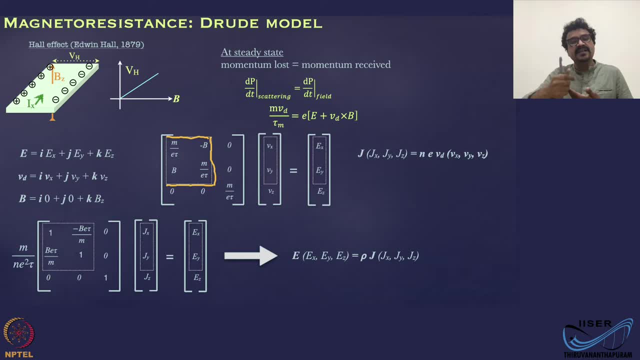 happens in the plane, whereas the direction along the field or parallel field is not going to get affected by the field. So there, you will not see anything In effect of field. ok, in that component. Now, when you have, as I tell, when you substitute, 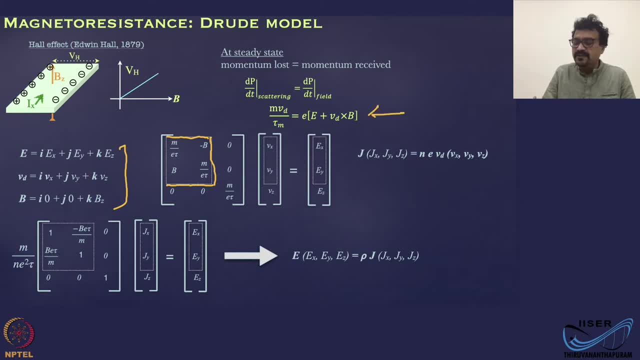 these equations into this equation, you will generate this matrix equation, and from this matrix equation you can this one by substituting J equal to N into BD. J is the current density, J has the components Jx, Jy and Jz and BD has the component Vx, Vy and Vz. Okay, So the aim here is: we need 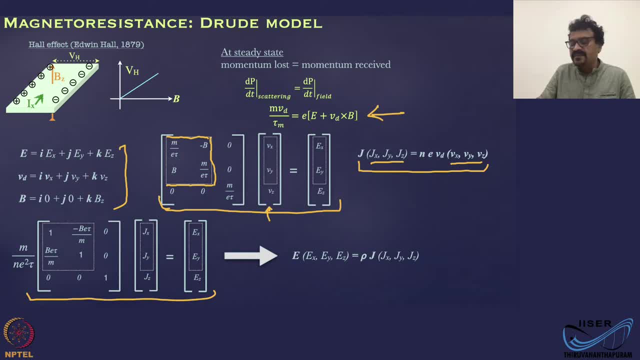 to replace this with the Jx, Jy and Jz component. That is only changed when you go from here to here. So here you take these Vs and replace those with Jx, Jy and Jz using this equation And you do some rearrangement and eventually you will get M by N square tau. Okay Into. 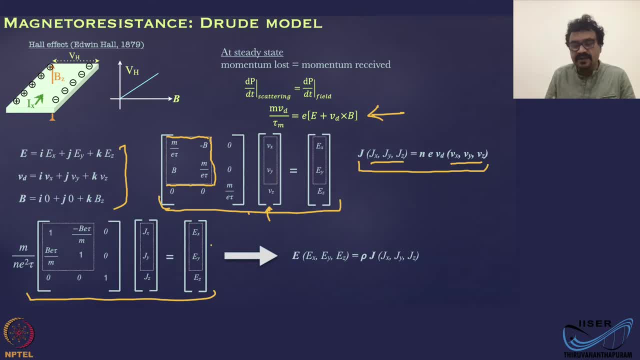 this matrix, the J matrix is going to give you the J vector, is going to give you the E vector, electric field vector, Okay, And this is basically equal to the formulation: E is equal to rho into J, that is the Ohm's. 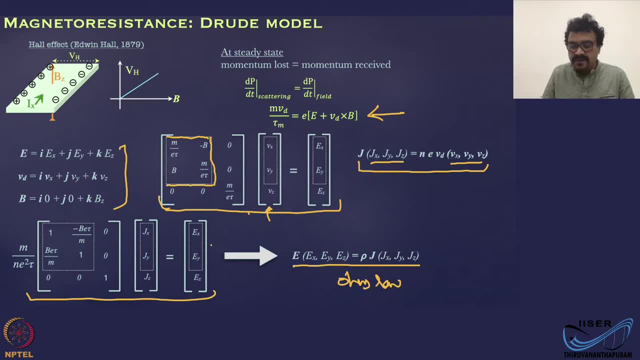 law. Okay, Where this rho is nothing but the restivity, J is the current density and E is the electric field. Okay, Because you are familiar with the Ohm's law in terms of the conductivity. but this is just restivity. So what you are familiar with is J sigma into E. Okay, And this is just. 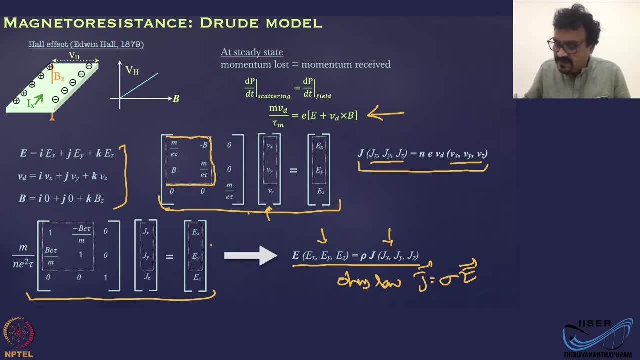 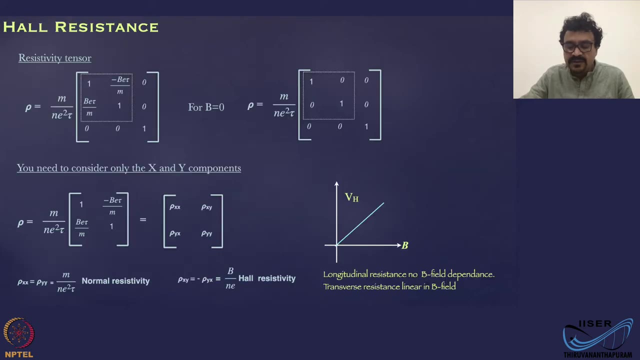 the sigma is replaced by E. Yes, One by rho, That is. then you take that rho to the other side. Okay, That is what it is. Okay, So here. what you have now is you have this rho, the restivity, as a tensor. It is a restivity tensor because it has components in all the direction. Okay, 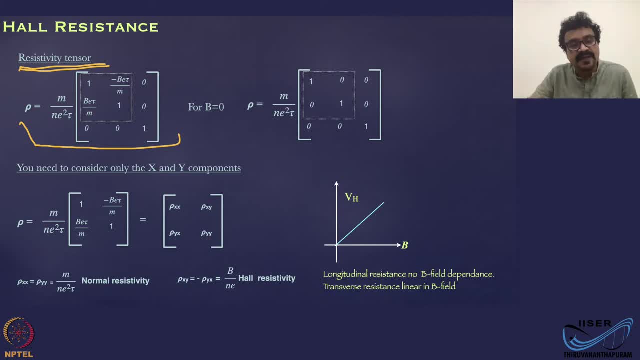 Okay, So it is a three by three. matrix m is m by n. square tau is the restivity when you do not have you have no b field, or when the b field is 0, and this is an isotropic quantity when you do not have any b field. 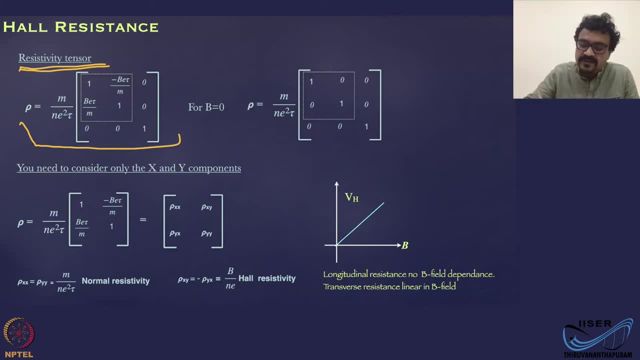 the moment you turn on the b field, you are going to get this of diagonal components. ok, those are proportion to b field of diagonal components. the diagonal ones are independent of the b field. now, as i told, the third row and third column, which represents the component which involves the z direction, we do not need to consider because field does not do anything. 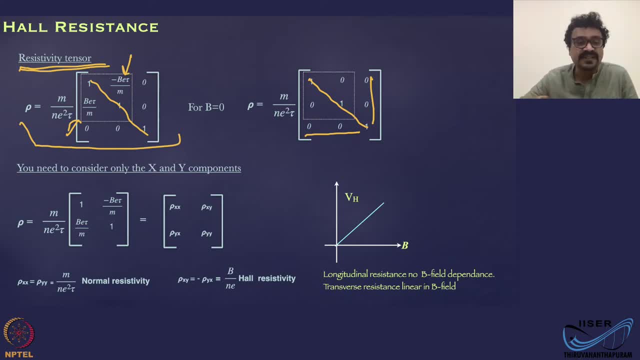 in that direction. the magnetic field does not do anything in that direction to the charge carrier. so for the time being, to ease the discussion, we can ignore that and we can just take the matrix which is the 2 by 2 matrix here and that resistivity is given by m, by n square tau into this matrix. 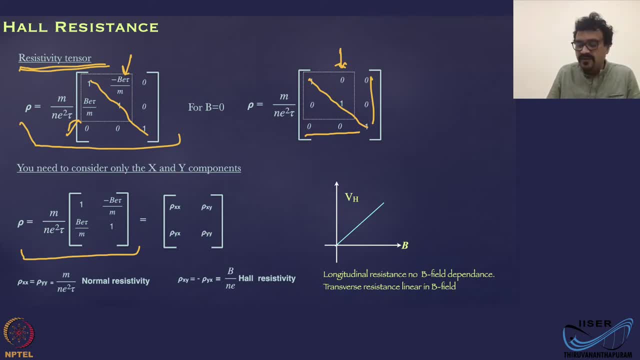 inside, and this is of the form you have: rho xx, rho xy, rho yx and rho yy. ok, this rho xy and rho yx, the of diagonal components, which involves magnetic field, and the diagonal components, which are your normal resistivity, which is equivalent to the, your ohm's flow. 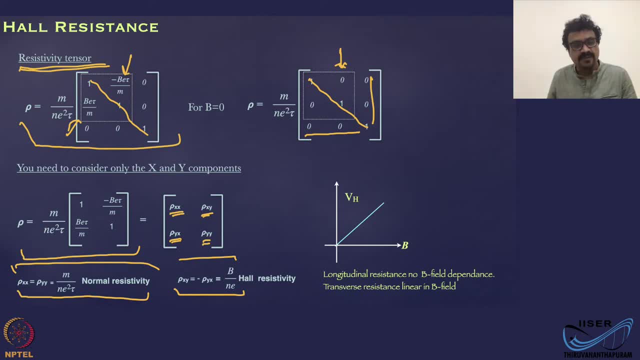 derivation using the classical drools theorem. this is the normal resistivity and the of diagonal components, the rho xy and rho yx, Z zeros are normal resistivity and if you include rah golaPro per Rec, the result that has to be X Super 128 times n times a. Φ will be a reverse. 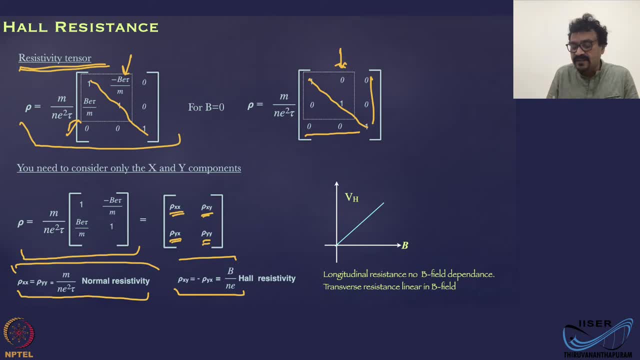 norm minus 1 magical harmonica in your 270 degree Thomist y x, the rho x y is negative of rho y. x is b by n e. that is the Hall resistivity. ok, and the Hall resistivity is proportional to b and it is inversely proportional to n. So 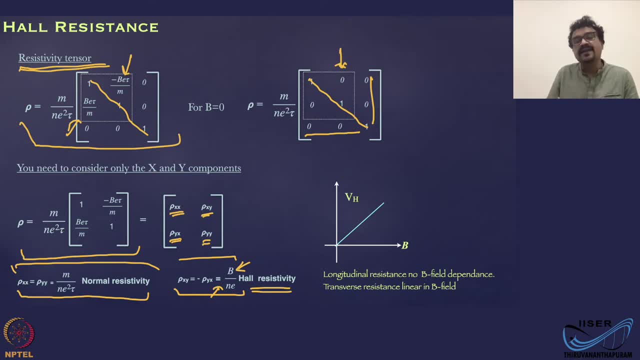 directly from this slope. you can calculate the carrier concentration from here. this is proportional. the Hall resistivity So v, h by i, that will give you the r, rho, x, y. ok, that is your Hall resistance. ok, Now, that is proportional, that the slope of that is proportional to. 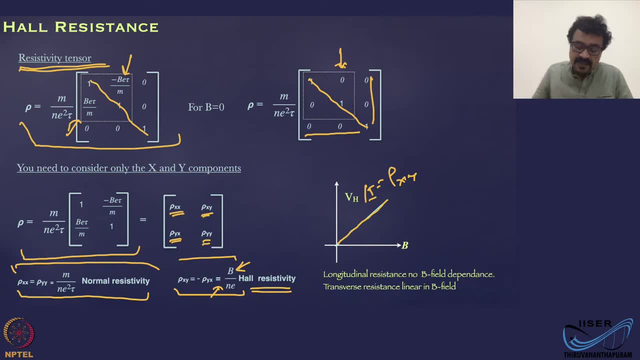 the b field. ok, but at the same time the longitudinal resistance does not have any dependence on the b, Whereas only the transverse resistance has a dependence. longitudinal resistance is the resistance along the propagation, along the direction of the applied electric field, and transverse is the one which is normal. perpendicular to that is the x- y term. If we assume the. 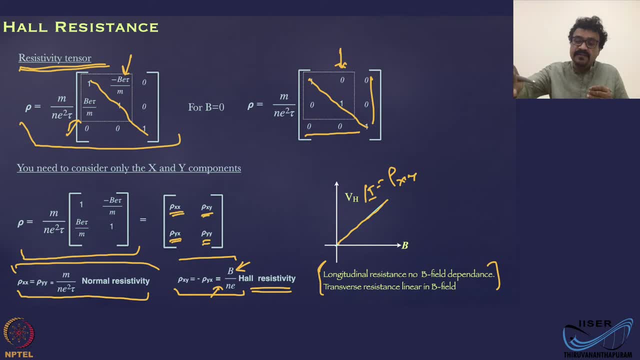 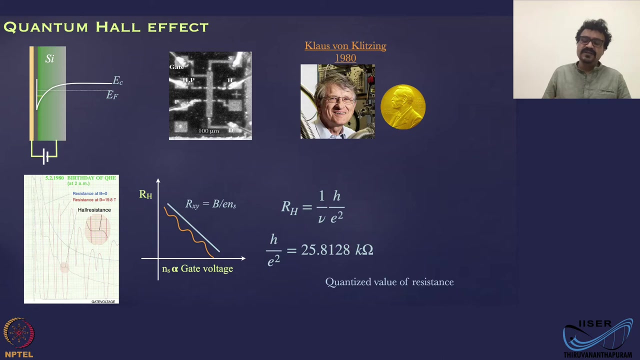 electric field applied in the x direction. magnetic field is a direction I am discussing, or I am talking about the x? y direction, the x y direction, that is proportionately b field, and this is the classical Hall effect. alright, Now, if you do this experiment, the same Hall. 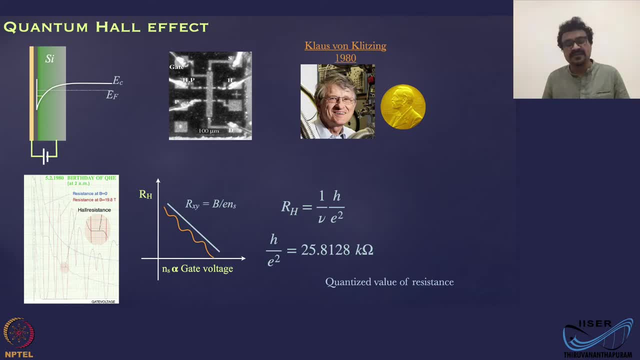 effect experiment, the 2 dimensional system, a clean 2 dimensional system. ok, when I say clean 2 dimensional system, just ample mean free path so that the electrons which are undergoing the cyclotron motion. 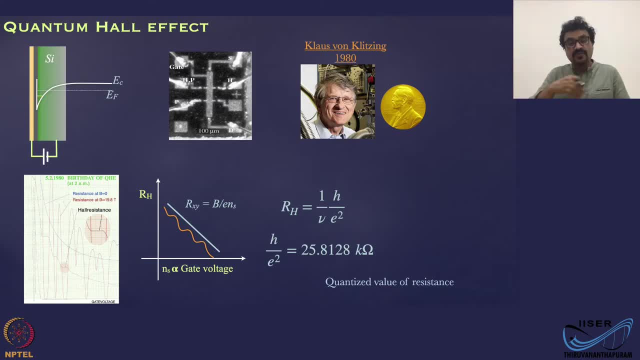 can complete the full, I mean full, full circle, at least one full circle. ok, now, if you do this experiment in clean system, you will the things in two-dimensional it's. a two-dimensional system is going to reveal a slightly different Hall effect picture. so that is the quantum. 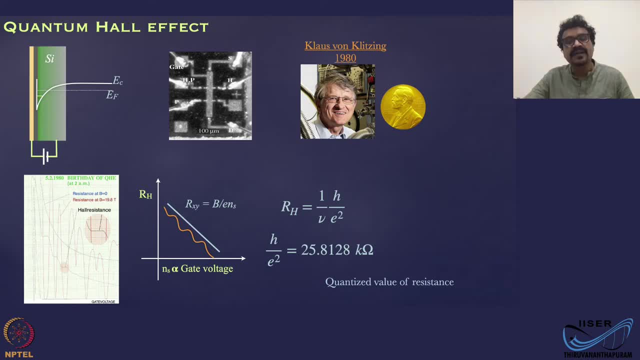 Hall effect. ok, that's about. that is a quantum mechanical counterpart of the Hall effect, so I will briefly review. I will give you an overview of what that effect is in this class. now, how that effect is used in certain technology is called a quantum electrical metrology. in quantum electrical metrology as a resistance. 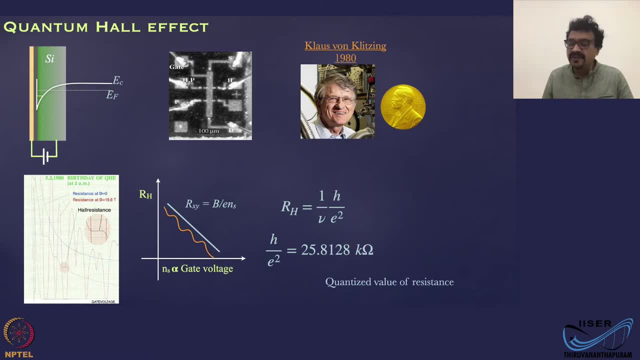 universal resistance standard. the quantum Hall effect was discovered by Klaus Wolclit Singh in 1980, which earned him the Nobel Prize in Physics. Thank you, Nobel Prize. So this is an extract from his lab notebook: Klaus Wolclit Singh lab notebook, which is: 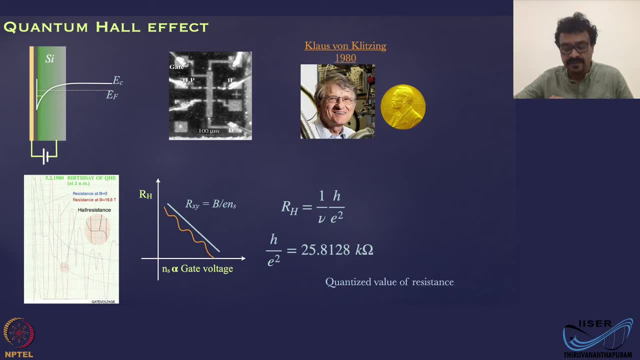 the birth of the quantum Hall effect. so here what we have is a silicon, silicon dioxide and metal. that is a some. it is a MOSFET, ok, and this, this is the top view of the MOSFET and this is the top view of Watt or spectrometer. 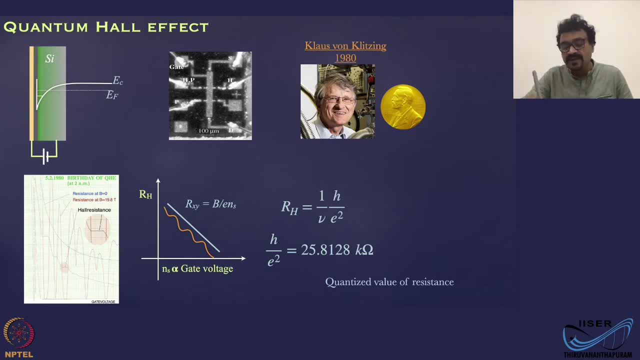 So, for the time being, what you can assume is: you have electrons or we have a charge carriers, whether we are seeing this lines or this bright regions, those are, those are the basically gates. you can think, ok, well, you have carriers in those regions. ok, so what do you have is when you apply voltage on to the gate and you have a silicon substrate, 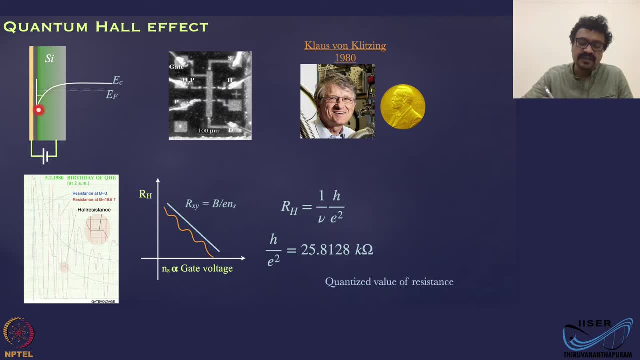 Ok, it is a MOSFET. you are going to create a thin accumulation layer which looks like a quantum well, which is actually a quantum well triangular shape, quantum well at the interface. You have charge carriers here. this is low energy region for electrons, your Fermi level. 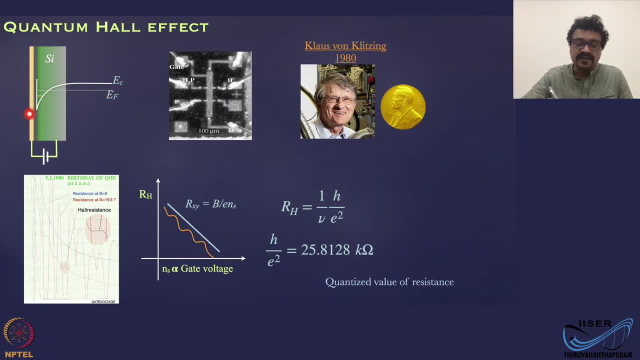 is somewhere here and you have triangular well and the well thickness or the width of the well is such that you have only one quantum level populated below the Fermi level. that is actually a two-dimensional system where the in the direction, in the z direction, which 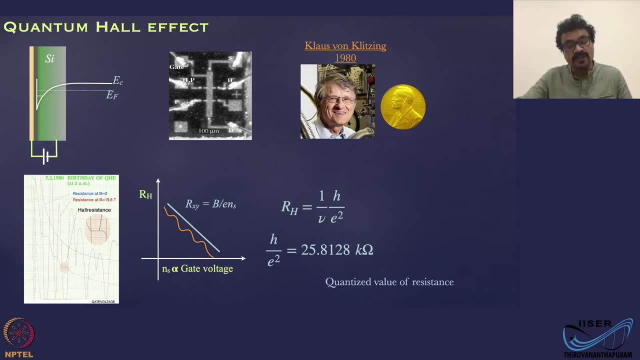 is perpendicular to the plane of this substrate. you have only one momentum state or there is only one k state. So then you can assume that that is a two-dimensional system. okay, But the charge carriers, as we discussed in the gallium arsenide aluminum gallium arsenide. 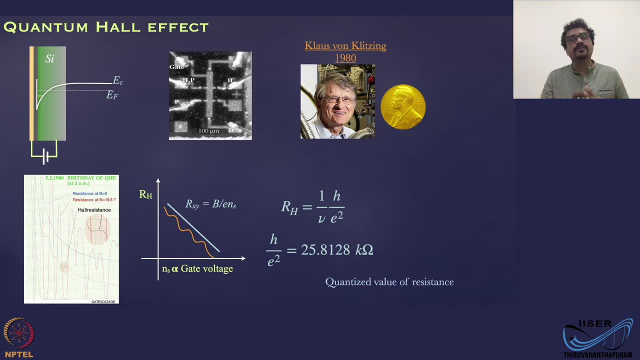 two-dimensional system. the charge carriers are free to move in the plane, but they cannot move, So there is no momentum state available for the charge carriers to scatter in the z direction. okay, Now the experiment is as follows: you have a B field which is applied. 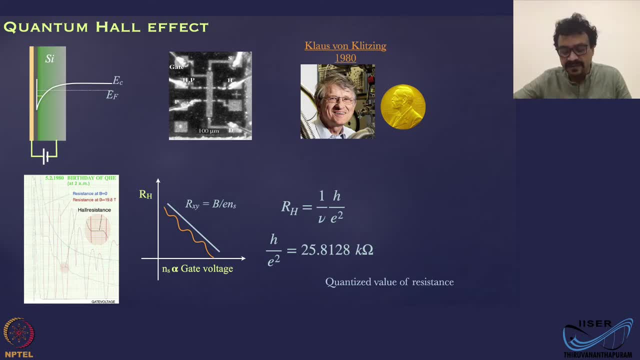 perpendicular to sample, perpendicular to this material, then what you do is you vary the gate voltage, which will change the charge density for carrier concentration in this well, okay, So you have, you have carriers in this, well, and you are going to change the 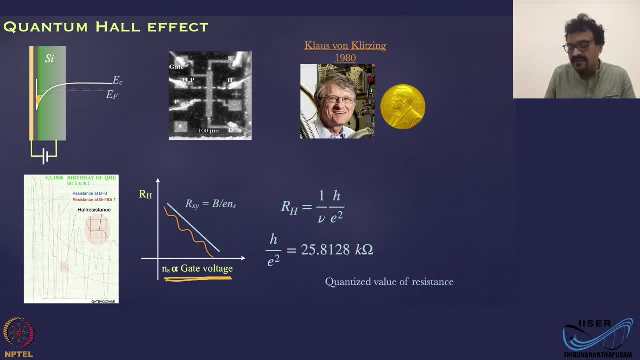 that carrier concentration, which I have labeled Ns, which is linearly related to the gate voltage. It is a- I think it is like a capacitor, where you are applying a voltage on this capacitor plate and the second plate of the capacitor is the two-dimensional electron system. So 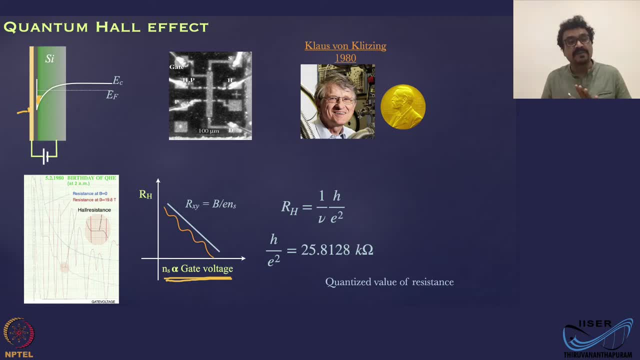 the number of electrons, which is the charge, can be multiplied by the number of electrons. Q on the capacitor plate is basically proportional to the voltage on the capacitor plate. okay, So that is the gate voltage. Now, usually, as far as Hall effect is concerned, the classical 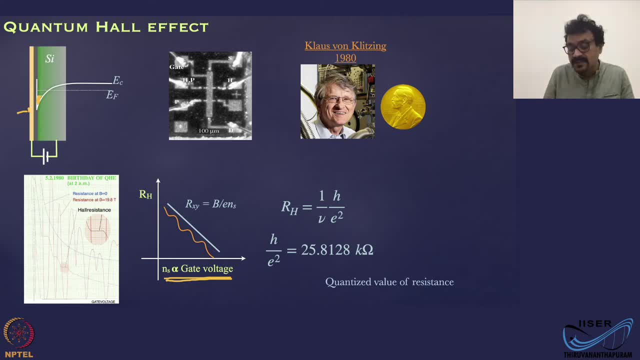 Hall effect is concerned. until this phenomena was discovered you have: Rxy is B by E into Nz. That means when you vary the carrier concentration by the gate voltage, there should be a reduction in the Rxy, which is the Rx, the Hall persistence. So what is expected as per classical physics? 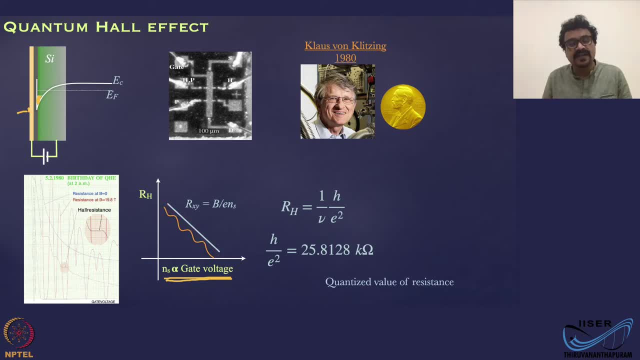 is this linear shaped straight line. okay, it is a straight line. Now what was observed is something like this: So if you look this graph carefully, let us focus on this curve, Let me try to draw on top of it. So this one. 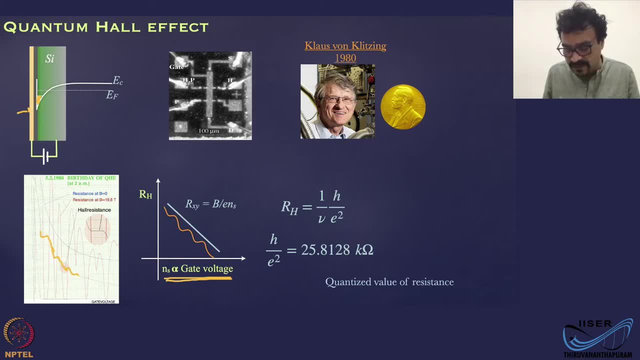 So if you look at this graph carefully, let us focus on this curve, Let me try to draw on top of it. So this one, When you have a step region of the step under step, this curve, okay, So I have kind of. 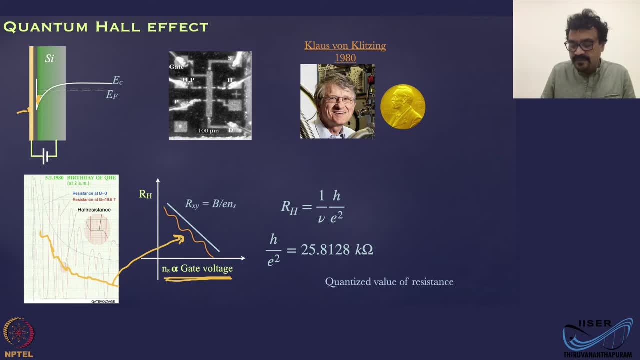 try to give you a feeling of what the curve is going to look like. Do you have flat? We have these steps shaped curve and this is a magnified view from that curve. okay, So let us draw on top of it. time, attack, range, charge, which is the result, The angle and numbers. 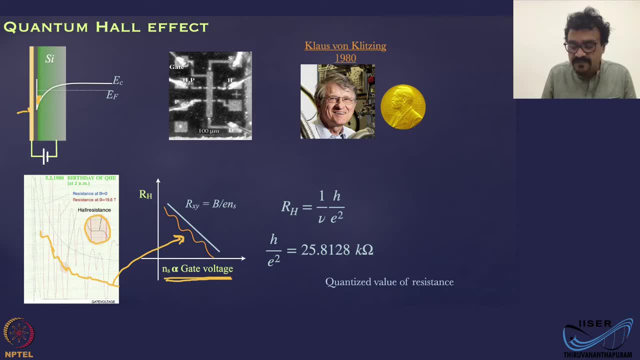 of At will change over time, but we did not test before that When you have a large Roman is a step as quantized, certain value, r, h, which are given by this formula, where nu is an integer. okay, so what we have is you have a step shape curve instead of a straight line, where the step 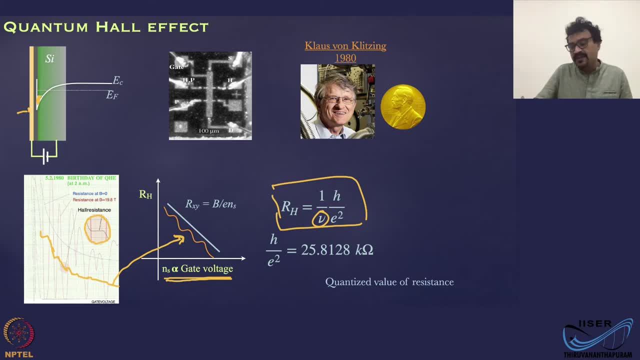 values are actually quantized in h by e squared. that means the the highest value is h by e square and the other steps are one by nu of h by e square. okay, but h by e square is the resistance quantum or quantized resistance value, which is equal to 25.8128 kilo. 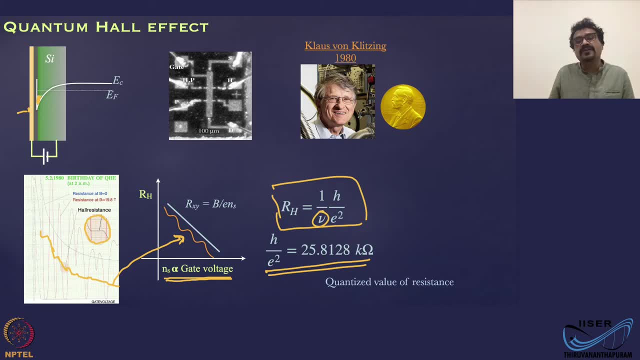 okay. so this is the quantum hall effect, where the all resistance is quantized in h by e square. i would say conductance is quantized because all resistance is one by nu. when nu is an integer okay, you say integer okay. so it is rhs quantized in one by nu. 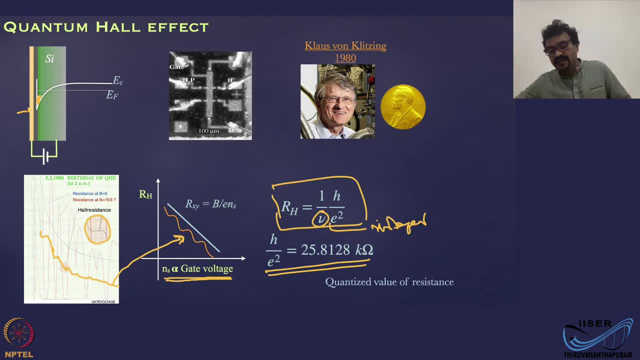 where nu is in this into h by e square. okay, this is the quantum heart. now, this was done in silicon mosfet geometry in silicon, at low temperature. okay, you can see that this is done at really high field, okay. and even what time is also marked. it's around 2 am, you know early in the morning. okay, we turn him. 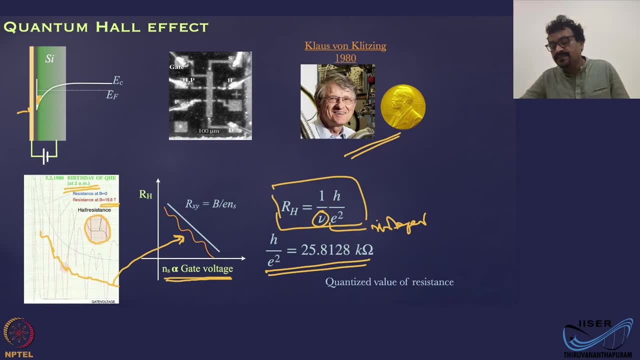 the number place in our place in physics. okay, this discovery happened in 1980.. now what we have from the previous slide is we are varying the rxy by varying ns, but instead of that you can also vary b field, the magnetic field. so the later generation, high mobility, generation of. 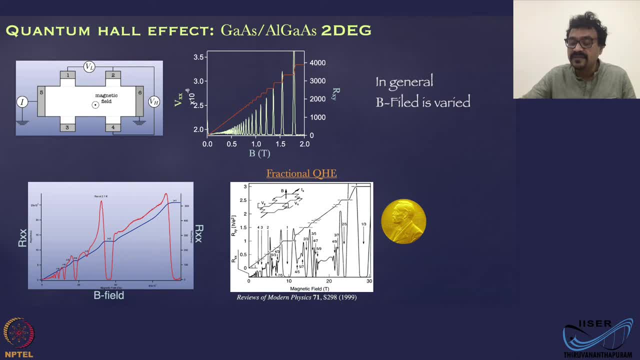 high mobility material based on the, the three, five, the gallium arsenide, aluminum, gallium arsenide or similar system. those are high mobility materials based on the three, five, the gallium arsenide, aluminum, gallium arsenide or similar system. those are remotely dropped. they already have carriers in the well, in the quantum well, the formation of the. 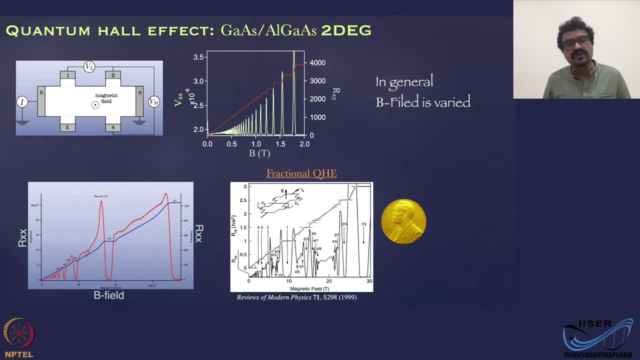 well, we have discussed extensively in one of those modules. okay, so you have again similar geometry where you are injecting current and you are measuring the voltage across or perpendicular direction of current. where is the where the magnetic field b is applied- perpendicular plane? okay, and this data is taken using one of those samples and what you are seeing here is the rxy, the whole resistance. 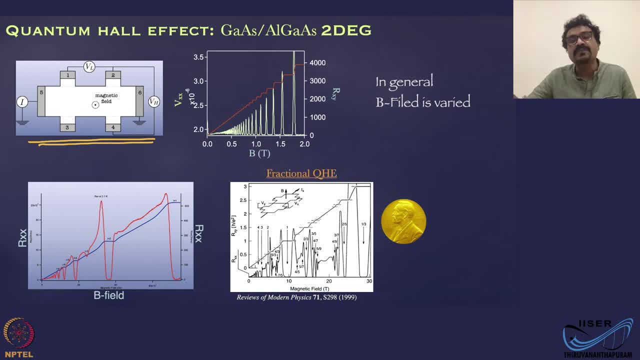 is showing a step like feature, as shown here. okay, this rxy. okay now, at the same time, you are also seeing a vehicle, a reaction that is taking place on top of the photothof. ok, red. next next, where the c direction of the field is called Sublikov-Dihasz oscillations, and this is the quantum Hall. 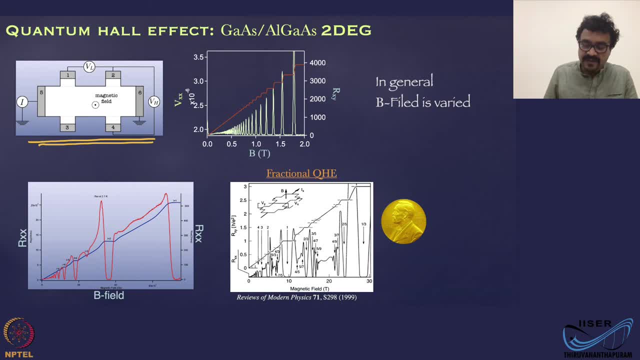 effect, the step-like feature in the Rxy and you can see this is one of the high field behavior. here is the low field behavior. okay, the high field behavior. you can see that you have plateau at you know any single loop, one, this axis you have to map back to here, this. 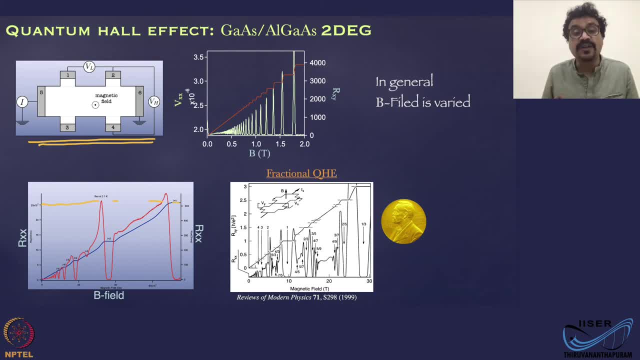 is the axis that is around 25 point. no, it's not around, it's actually exactly 25.8138. and the second one is here, half of it, and third one is here and so on. okay, and there are also oscillations: the red shaped, red colored curve. 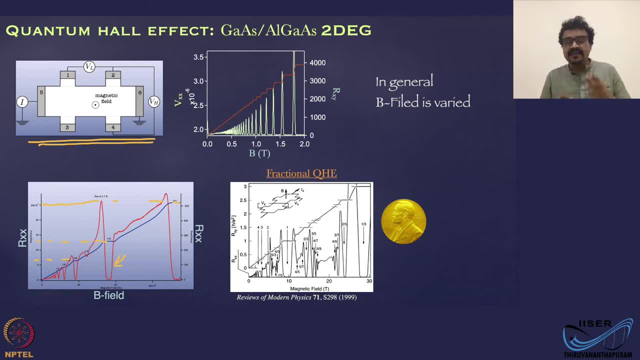 in the Rxx, that is, the linear resistance, or resistance along the direction of the field. so if I mark it here, Rxy will be this and Rxx will be the resistance in this direction. okay, the direction in the direction of the field, electric field- okay. 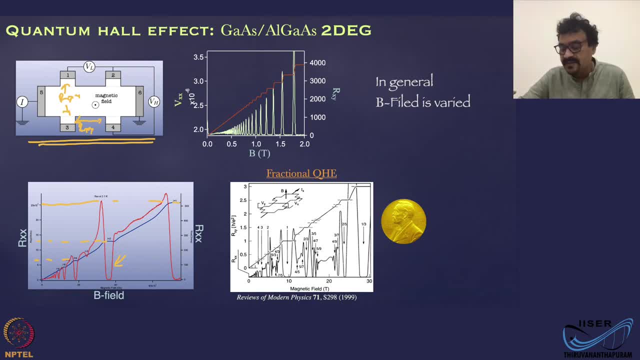 Now, a few years later, as the technology of making higher and higher mobility material got matured, the experiments start observing a slightly complicated, intricate Hall effect that is called fractional quantum Hall effect. okay, In this case. In this case, you have plateaus, or flat regions in the Rxy, but not only at integer values. 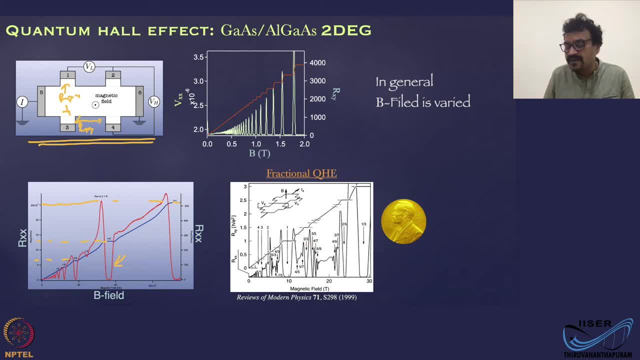 but also at various fractional values, as marked here. this, if time permits, we will try to discuss in one of the classes, but this is not going to be discussed in detail anyway in this course, which is beyond the scope of this course. okay, But this is called fractional quantum Hall effect, where you have resistance quantized. 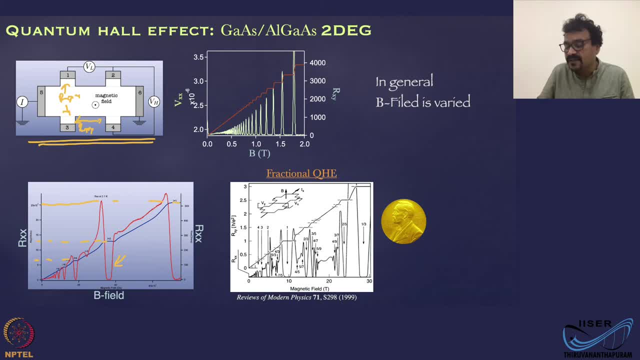 at fractional. So you have two values, certain fractional values at 1 by 1, third, 2 by 7, third, you know 9 fourth, and all these values okay, which are marked here, that earn a second noble prize for the quantum Hall effect phenomena. okay, the first one was for integer quantum Hall. 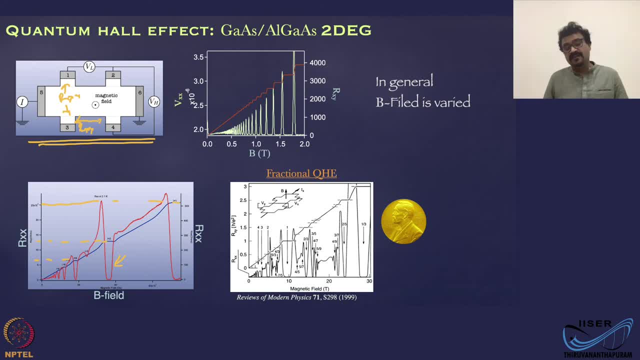 effect. the second one was for the fractional quantum Hall effect, and this is a very fascinating phenomena, Because physics is kind of very different from that of the integer quantum Hall effect. So, to put it briefly, integer quantum Hall effect is something which you can explain. 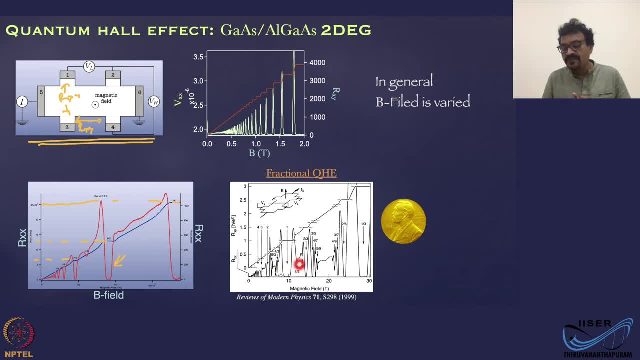 using single particle picture, but fractional quantum Hall effect is a many body phenomena. okay, There are fractional states, there are composite particles. here you have electrons, but in this case you have composite particles. okay, so that is a many body phenomena, but this one you can explain with the single particle picture, okay, and that we will explain during this. 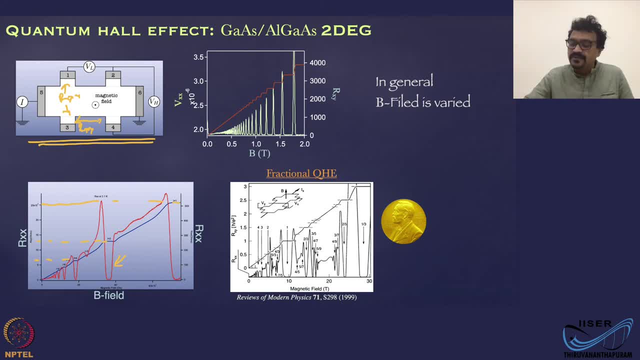 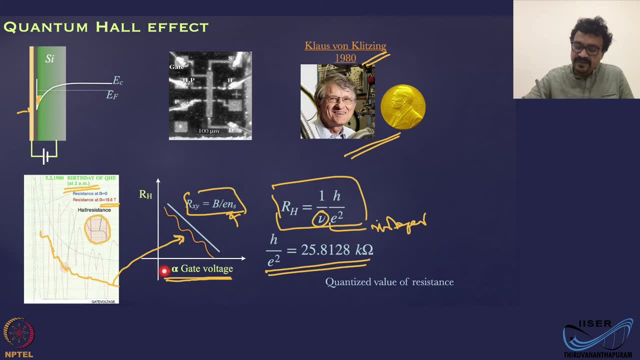 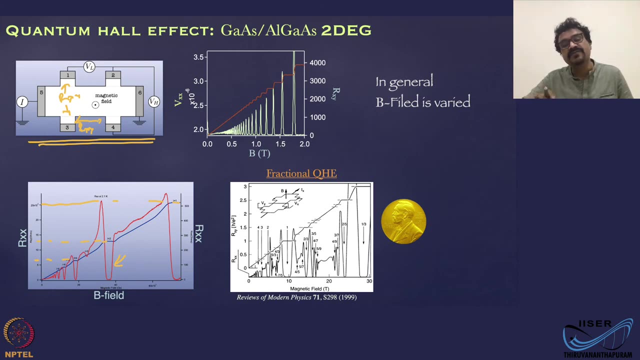 course, okay. Now the difference here is: in this case we have varied the carrier concentration by fixing the B field. in this case we have fixed the carrier concentration but varied the B field. but anyway, the ratio between the magnetic field and the carrier concentration is what we have varied. okay, 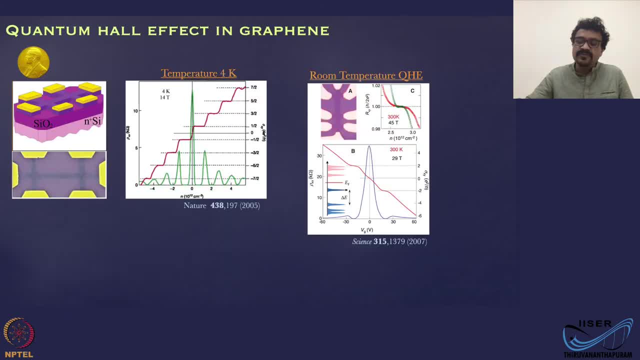 Now the advent of the new generation two-dimensional systems, the first one being the graphene. it is a sheet of carbon atom and one of the first experiment after extraction of a sheet of carbon atom, So after extraction of sheet of carbon atoms from graphite, is the magnetotransport where 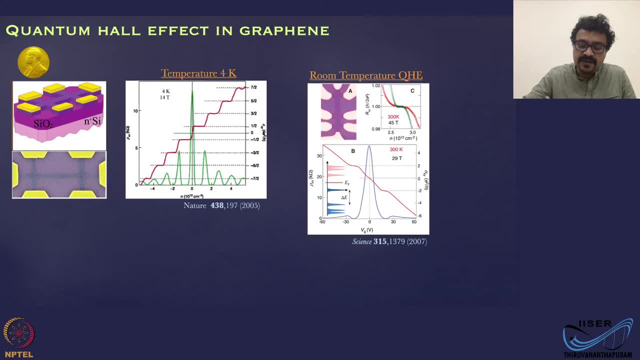 you apply a magnetic field perpendicular to plane of the sheet where you have a back gate which is highly doped silicon and there is a silicon dioxide gate oxide. then you have the sheet. of graphene then is patterned to form in the form of a Hall bar. this is the 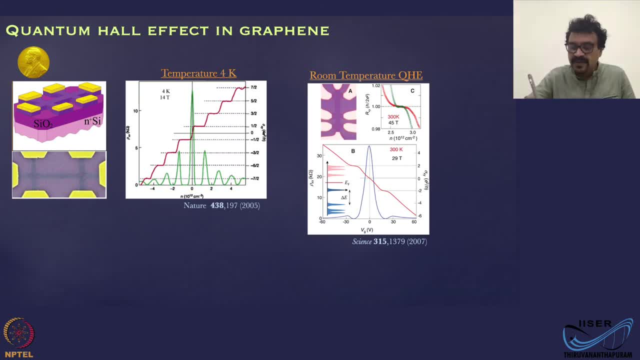 top view of that, okay, Okay. And when you conduct the same experiment where you measure the transverse resistance as a function of magnetic field over carrier concentration? so in this case the magnetic field was fixed at 14 tesla and the carrier concentration was vary by varying the gate, the back gate. 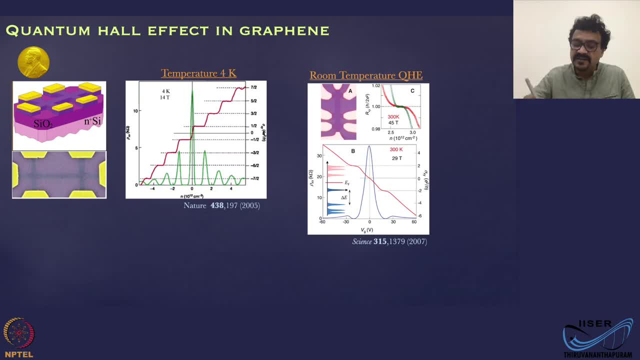 okay, When this experiment was done. Okay, Then also, they observed a step like feature as opposed to a straight line in the Hall effect and of course, they also observed oscillation in the rxx, that is the green color here. This experiment was done at four color, okay. 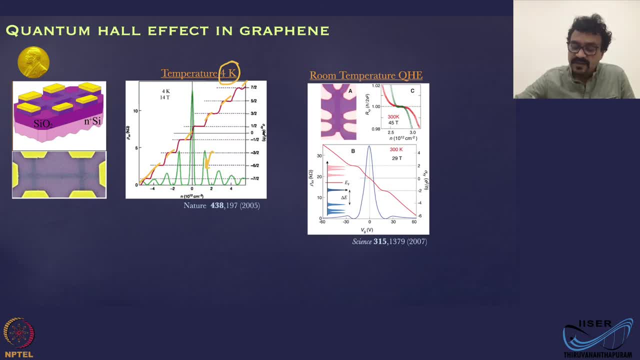 Now this red color trace: Okay, This red color trace, Okay, This red color trace represents the Hall resistance and that also shows step like feature and is quantized. if you look at carefully, the unit here is 4 e square by h. okay, instead. of. 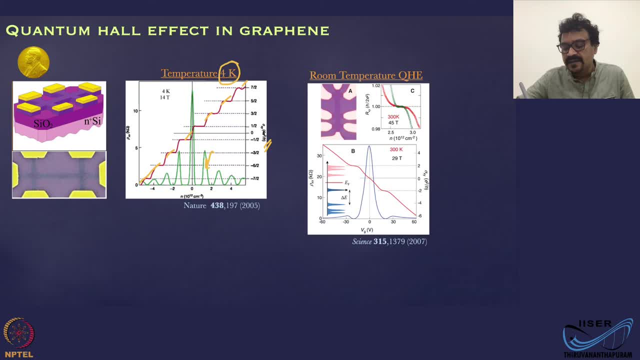 e square by h, and the detail physics, if time permits, we will discuss, but that has to do with the nature of this charge carriers. those are not the normal conduction and electrons that you find in these kind of free electron gas. Okay, The silicon free electron silicon or gallium arsenide material. here you have a direct 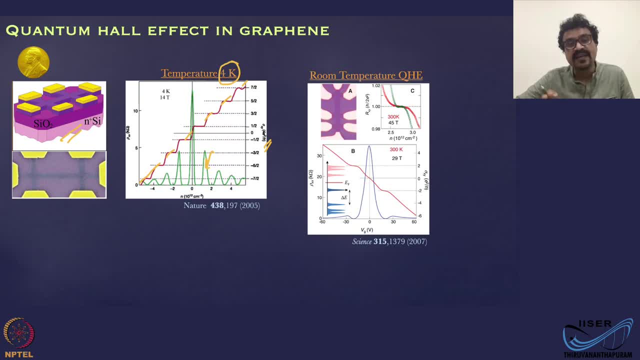 particle, massless fermions, and you have valleys and you have spin degeneracy, that all these, because this is done at a really high field, all this together is going to give you a slightly different Hall effect, but still it is quantized. the resistance is Hall resistance. RH is quantized. 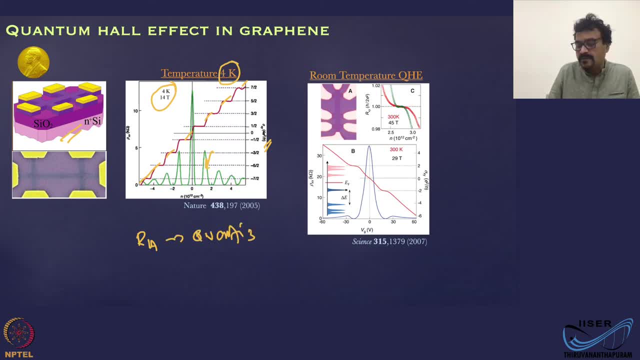 that is the point, Okay, It is quantized in this picture also and, surprisingly, this effect was observed even at room temperature. okay, you can find more details about these in these two papers. okay, and I would say that is probably. I can say it is a third Nobel Prize for quantize, though it is not directly. 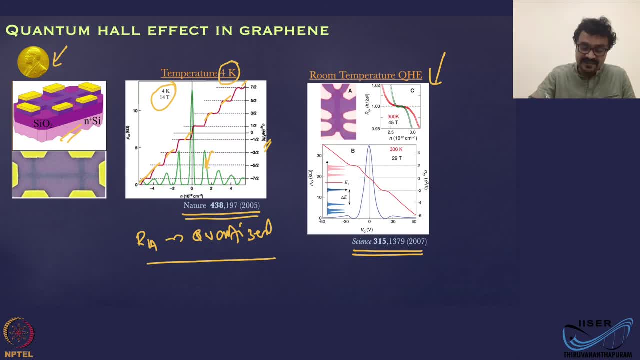 for quantum Hall effect: Okay, But the feature that demonstrate in this experiment is the quantum Hall effect- Okay. It is probably a third Nobel Prize for performing a quantum Hall effect experiment and interestingly, you can see this quantization even at 300 Kelvin room temperature in a sheet of graphene. 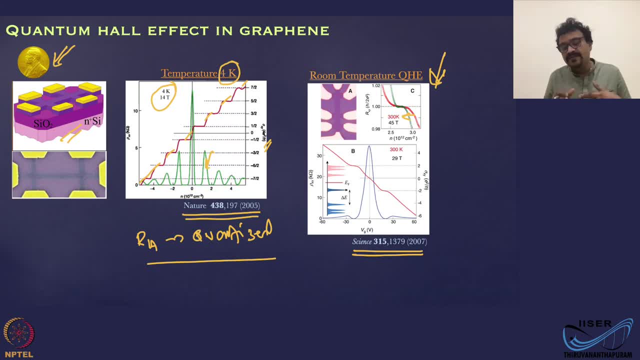 that is also okay. So what do you have Now? You have seen this effect in starting from a silicon MOSFET. then you move on to gallium arsenide structure, two-dimensional electron system. there also you saw same effect. and now there is another, completely different two-dimensional system. it is radically different. 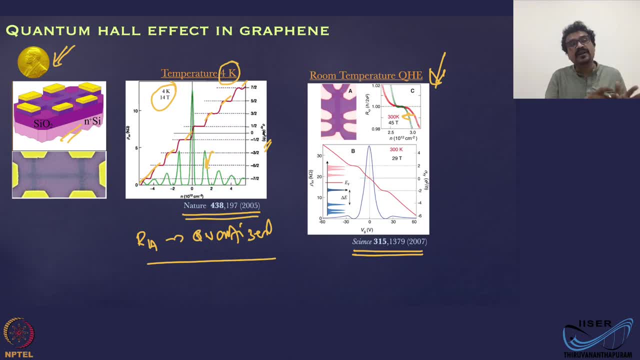 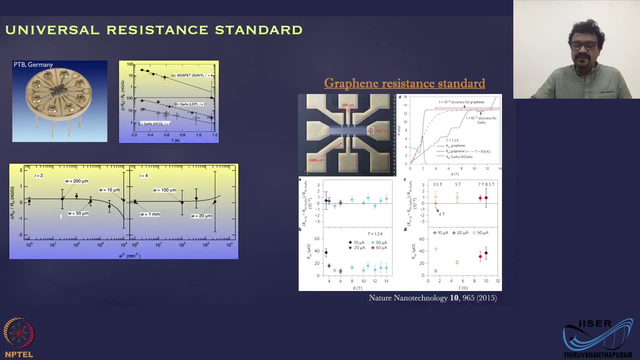 those are bulk two-dimensional system or interface in the bulk material- the first two ones- but this is actually a sheet, A pure sheet of atoms. there also you are seeing the same effect, the quantization, and it is so robust. so what we now need to realize is this: quantum Hall effect is a universal 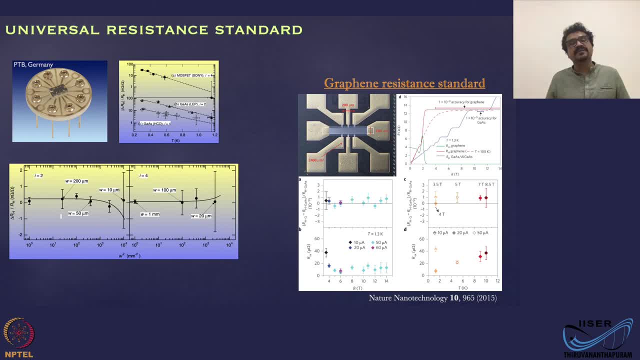 phenomenon. it does not depend on material system- okay. it does not depend on the kind of equipment you use- Okay. It does not depend on the temperature. as long as certain energy scales are met, you will see this effect. So, and this was initially proposed and now this has been widely well accepted and followed. 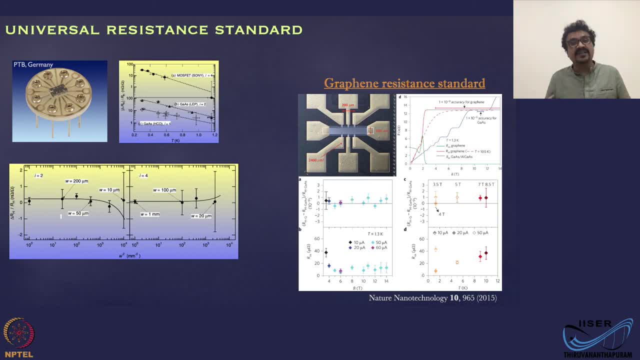 as a resistance standard, universal resistance standard in quantum electrical metrology. So this is a picture of one of those samples. It is a gallium arsenide sample, but this has been done on various materials and verified across the world, across the countries, that this is such a robust phenomena and the plots 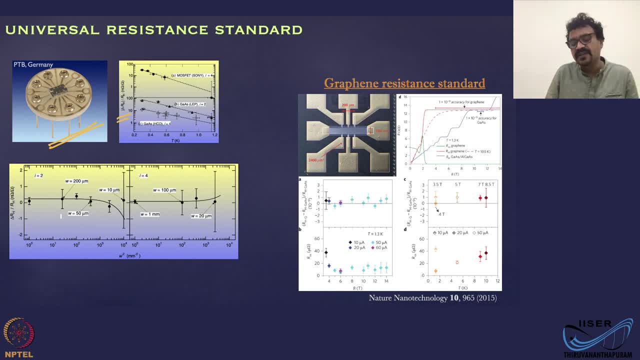 here are the errors that are measured in this: quantized values of resistance. those are in nano ohms. okay, at nine place after the decimal. okay, all these are in nano ohms. if you read the axis carefully, These are all error. that has been where variation that has been measured over various systems. 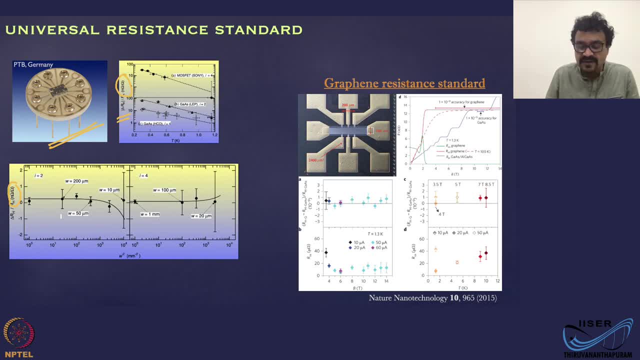 this is not even like one nano ohm, okay, one. this whole scale here is like three or four nano ohms, okay, Now, in this case, okay, so here is a 200 micrometer wide device. this is like 50 micrometer. this is a 10 micrometer, okay, and this is how the I is equal to the second plateau. 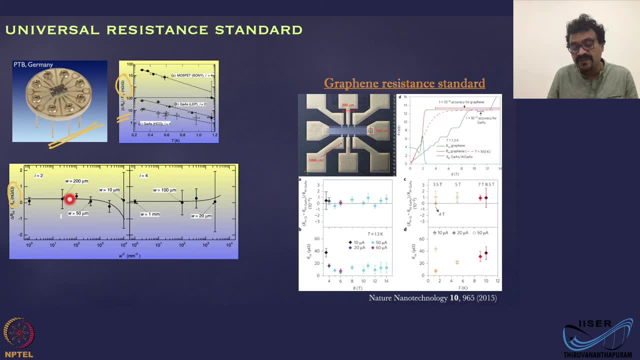 It was positioned and the error between various devices. here. this is also this, the fourth plateau, where error across various devices is in nano ohms. okay, Similarly, here these are done for various materials like gallium arsenide, as by various labs, and that is their error bar, overall error bar across all the devices. 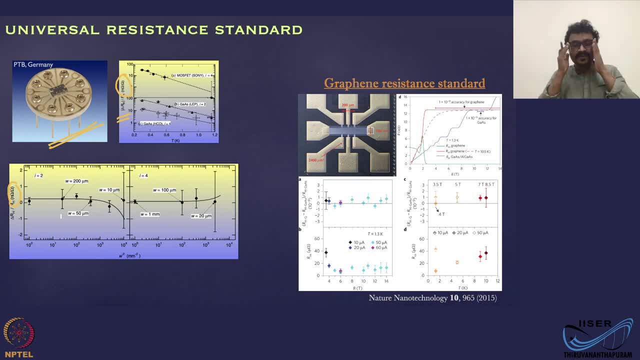 So this is the error bar. So this is the error bar. So this is the error bar. This is the error bar that I see here. This is the error bar for my macrospace. okay, That is in nano ohms. That is nine place after the decimal, such a robust phenomena, which is there is nothing.